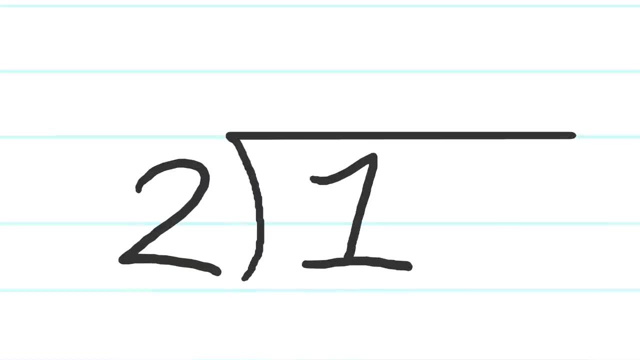 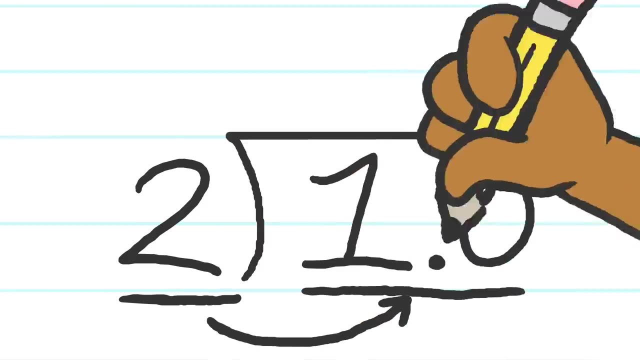 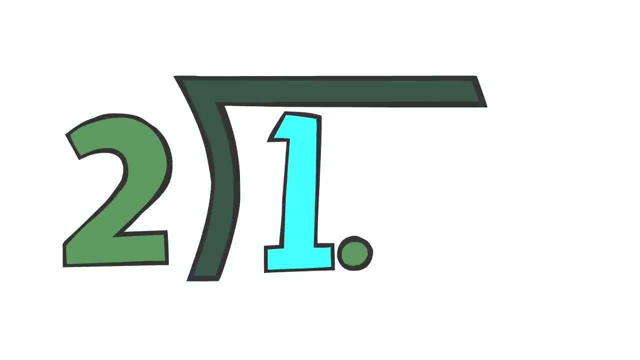 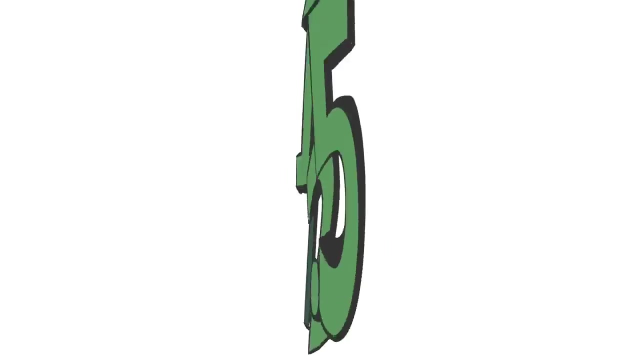 He said: listen, here's what you need to know. Just write a decimal point followed by a zero, And you know, two goes into ten five times. Then the decimal point rises above the line. The numerator becomes a dividend. Then write a decimal point and a zero in the tenths. Divide and write the decimal point in the quotient, So one, half and five tenths are equivalent. 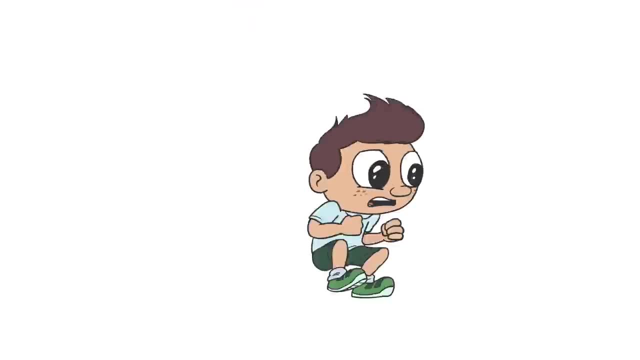 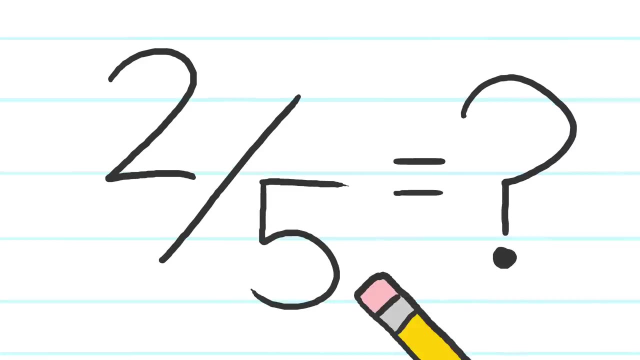 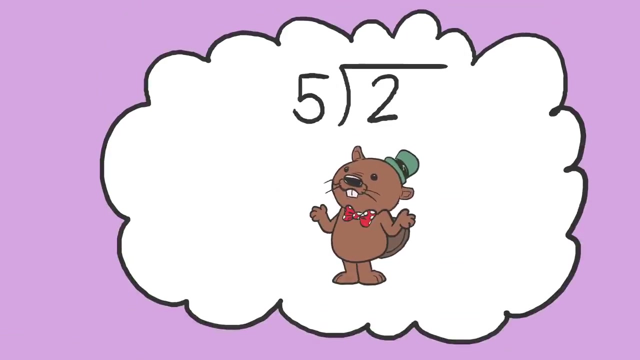 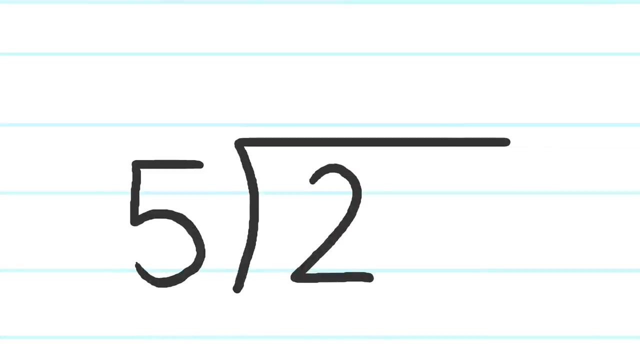 Later on I was hanging with my stuffed animal, Showing him how to convert a fraction to a decimal. I divided the numerator by the denominator. As he sat there real quiet like a spectator, I bet he was thinking five can't go into two. But luckily for him I knew just what to do. I said: listen, here's how it's got to go. Just write a decimal point followed by a zero. 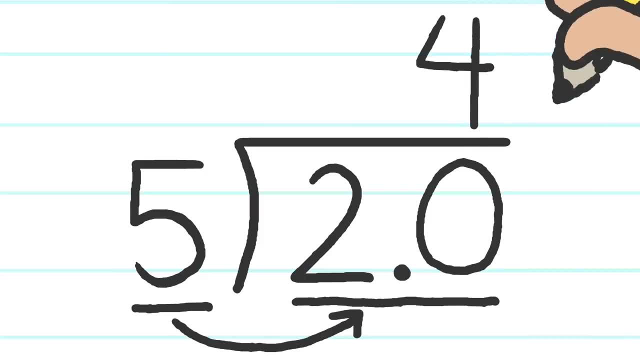 Then five goes in. So I asked: huh Well, how can that be done? He said: listen, here's what you need to know. Just write a decimal point followed by a zero, And you know, two goes into one. Then the numerator becomes a dividend. 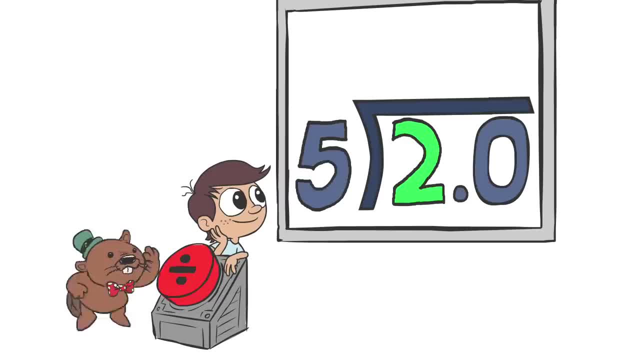 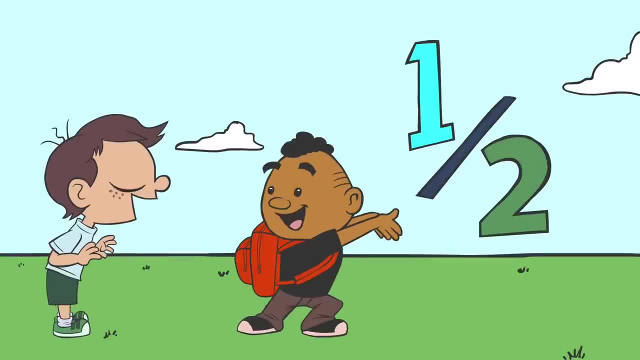 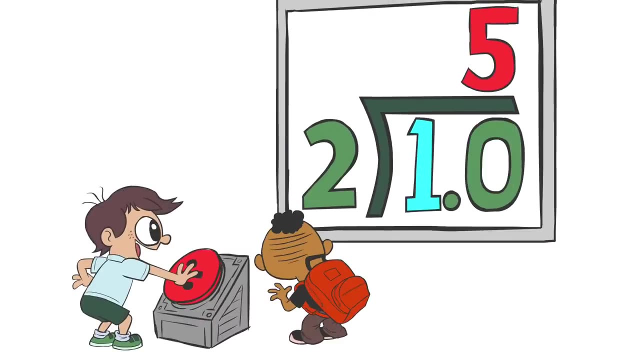 Then write a decimal point and a zero in the tenths. Divide and write the decimal point in the quotient. So two fifths and four tenths are equivalent. The numerator becomes a dividend. Then write a decimal point and a zero in the tenths. Divide and write the decimal point in the quotient. 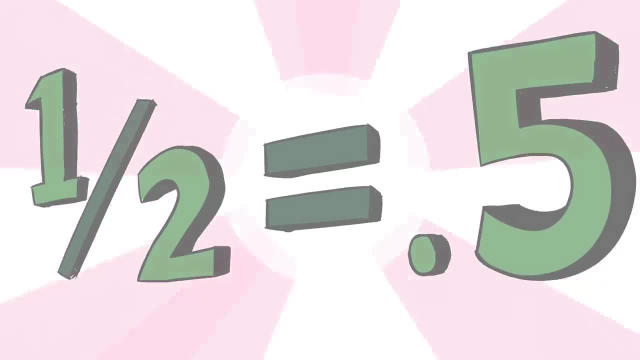 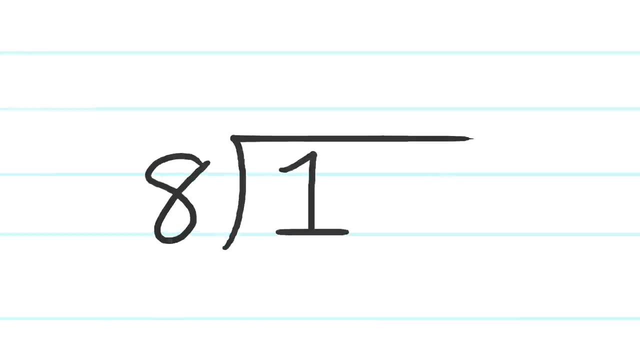 So one half and five tenths are equivalent. I had to get my homework done before the school dance. I had to convert a fraction, Couldn't leave it to chance. I divided the numerator by the denominator, But to my surprise there was a remainder. 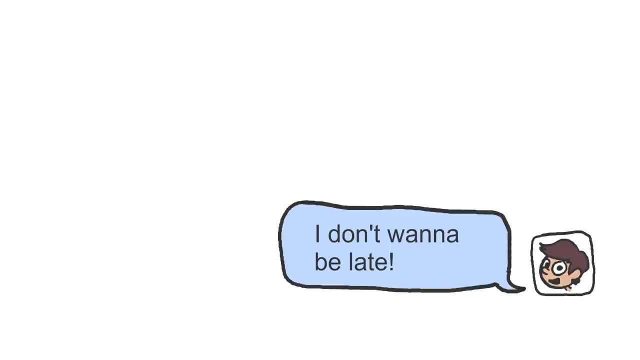 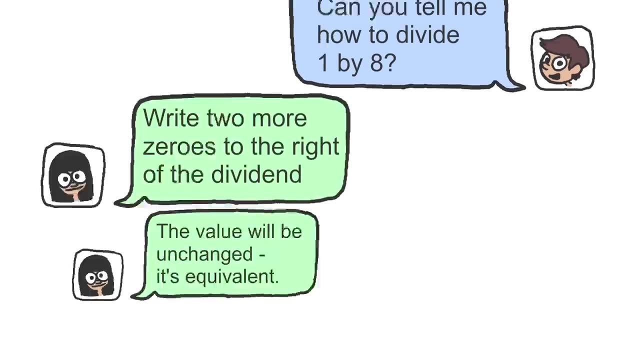 I texted my friend. I don't want to be late. Can you tell me how to divide one by eight? She said: write two more zeros to the right of the dividend. The value will be unchanged, It's equivalent. I divided the two numbers and got point one. 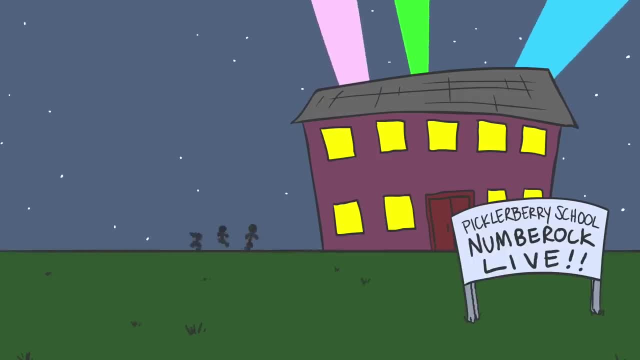 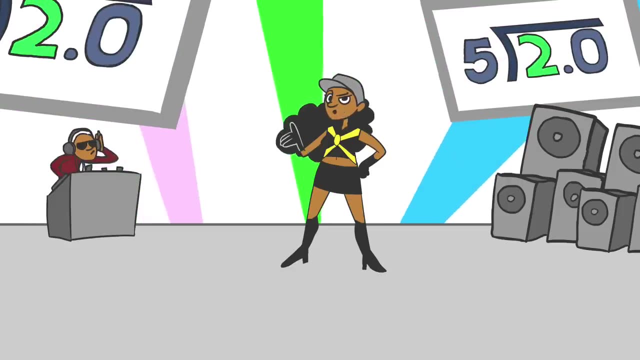 One, two, five. we arrived Just in time to see number off live. The numerator becomes a dividend. Then write a decimal point and a zero in the tenths. Divide and write the decimal point in the quotient, So two fifths and four tenths are equivalent.